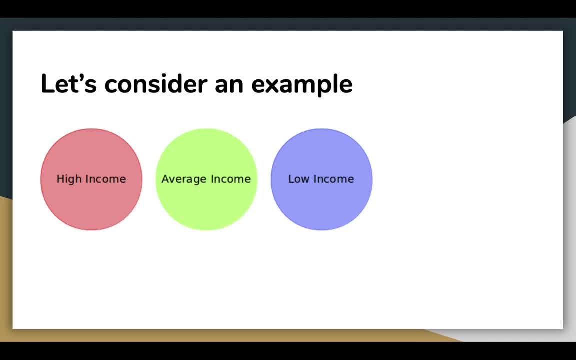 of each customer separately and then make a decision? Certainly not. It is a manual process and will take a huge amount of time. So what can the bank do? One option is to segment its customers into different groups. For instance, the bank can group the customers. 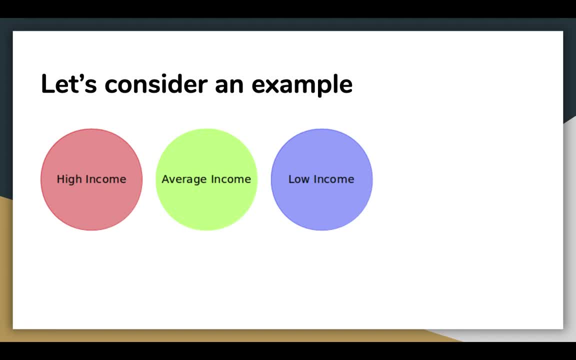 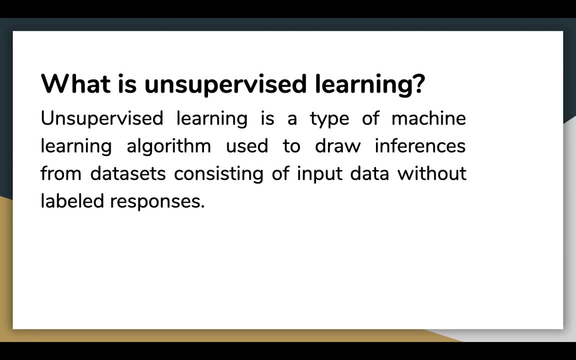 based on their incomes. The groups that are shown here are known as clusters, and the process of creating these groups is known as clustering. Awesome, Now let's talk about unsupervised learning. Unsupervised learning is a type of machine learning algorithm used to draw inferences from datasets consisting of input. 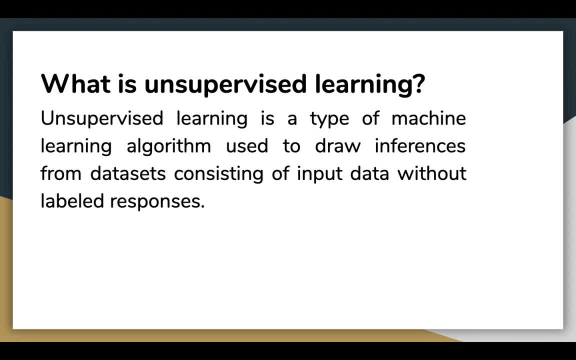 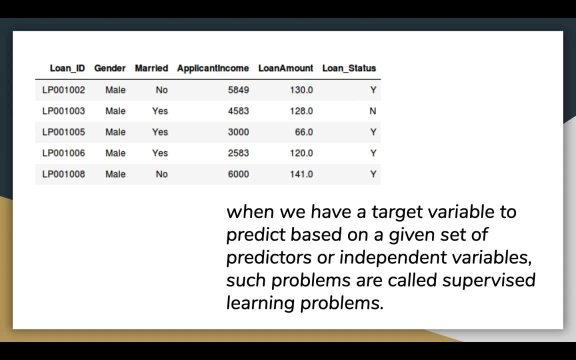 data without labelled responses. So to understand all of this, let's see how a supervised algorithm works. first, We have a labelled dataset with the output, or target variable. In this particular example, the task is to predict whether a loan will be approved or not. 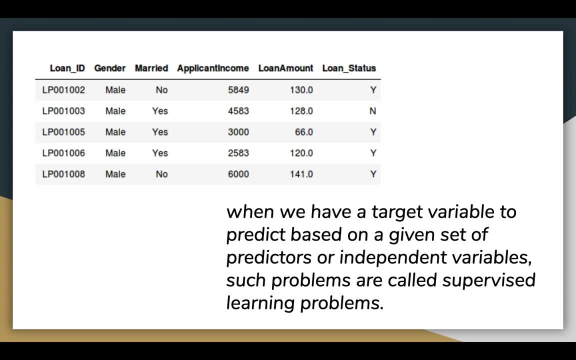 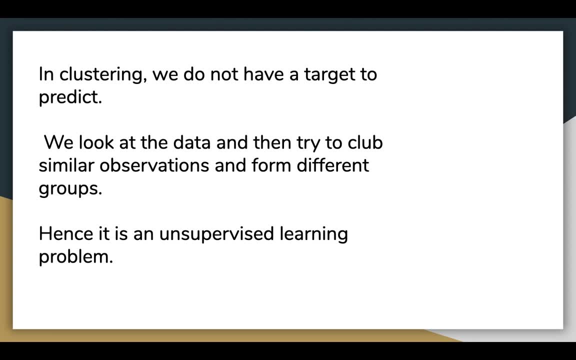 As we have all the data labeled with appropriate targets, we call it as supervised learning. In clustering, we do not have a target to predict. We look at the data and try to club similar observations and form different groups. Hence it is an unsupervised learning algorithm. 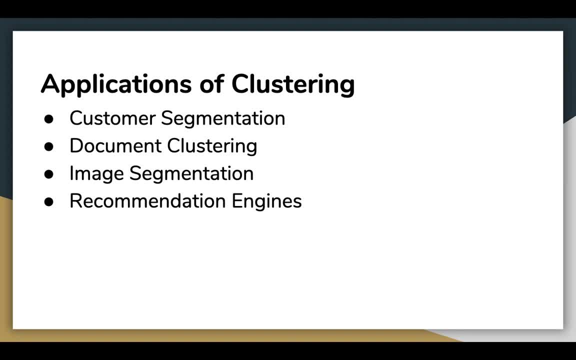 So let's see where this helps us in the real world. So, starting with customer segmentation- as we discussed before about the bank making clusters based on the income for the credit cards- Next thing is document clustering. This is another common application. Let's say you have multiple documents and you need to cluster similar documents together. 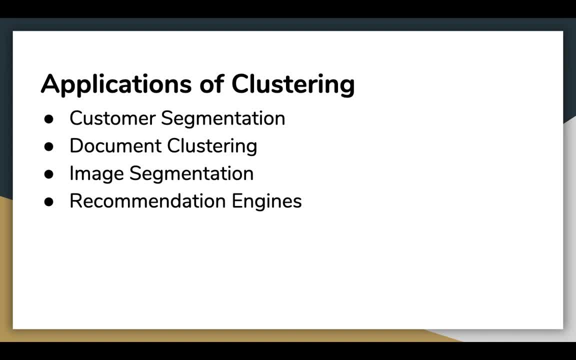 Clustering helps us group these documents such that similar documents are in the same clusters. The next is image segmentation. We can also use clustering to perform image segmentation. Here we try to club similar pixels in the image together. We can apply clustering to create a cluster. 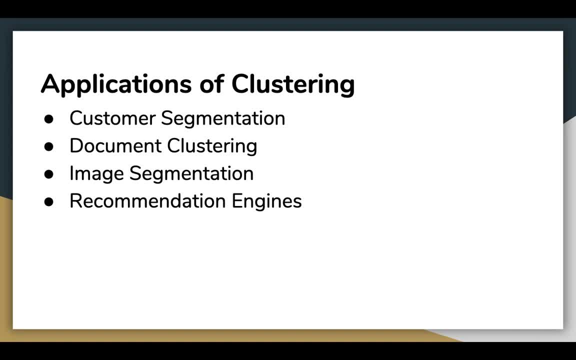 We can create these clusters having similar pixels in the same group. The next is recommendation engines. Let's say you want to watch or you want to recommend songs to your friends. You can look at the songs liked by that person and then use clustering to find similar songs. 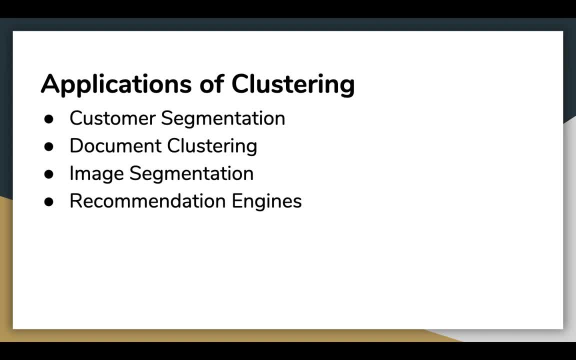 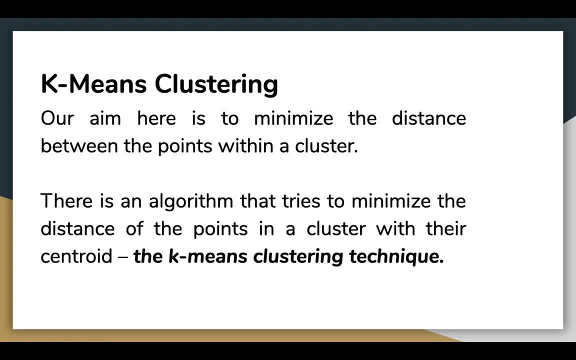 and then finally recommend those songs to the person. So let's talk about k-means clustering. now We have finally arrived to the main part of the video. Now, with regards to generating clusters, our aim here is to minimize the distance between the points within a cluster. 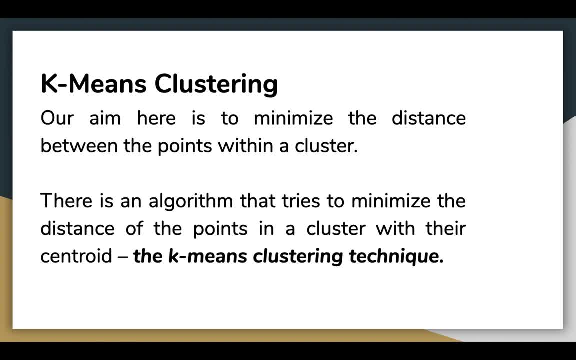 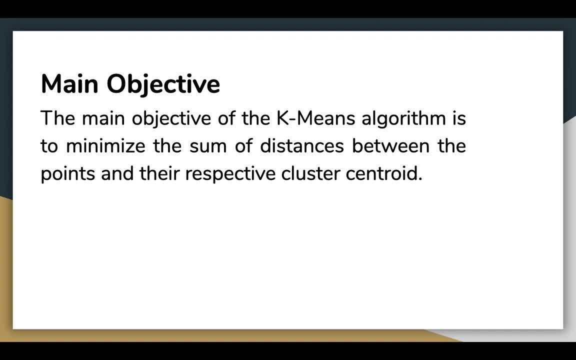 There is an algorithm that tries to minimize the distance of the points in a cluster with their centroid. This is called the k-means clustering technique. The main objective of the k-means algorithm is to minimize the sum of distances between the points and their respective cluster centroid. 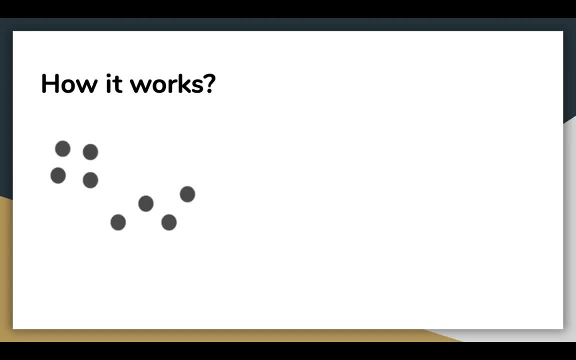 Let's see how the algorithm works in action. Let's see how the algorithm works in action. So we have these 8 points we want to apply k-means on to create clusters. So let's see how we can do that. The first step in k-means is to pick the number of clusters, k. 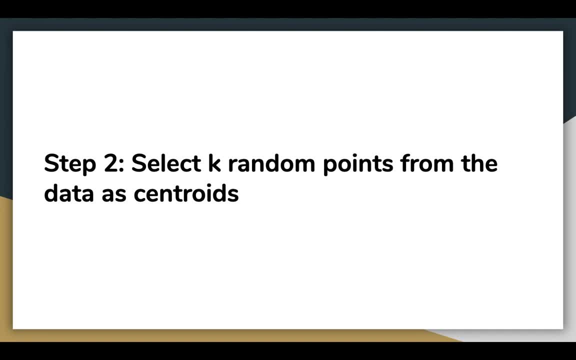 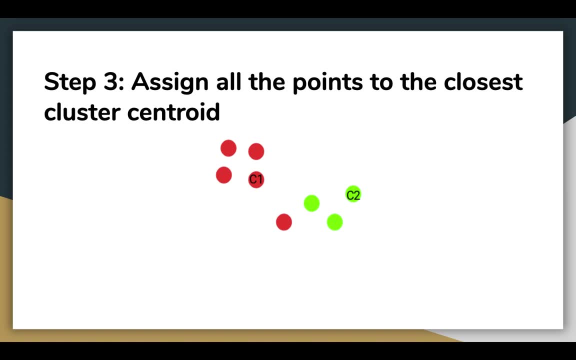 Next we randomly select the centroid for each cluster. Let's say we have 2 clusters, so the k is equal to 2 here. We then randomly select the centroid, Step 3. Once we have initialized the centroid, we assign each point to the closest cluster centroid. 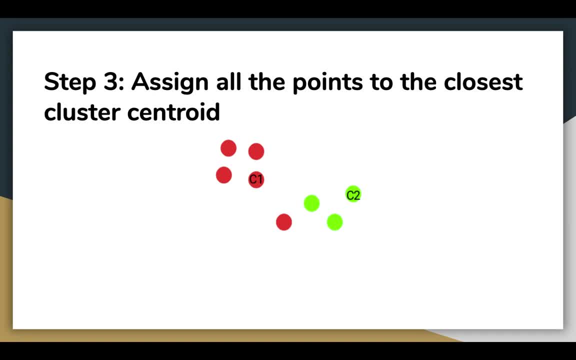 Here you can see that the points which are closer to the red point are assigned to the red cluster, whereas the points which are closer to the green point are assigned to the green cluster. Now, once we have assigned all of the points to an either cluster, the next step is to 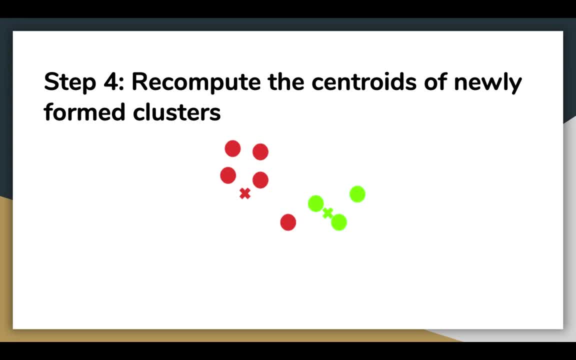 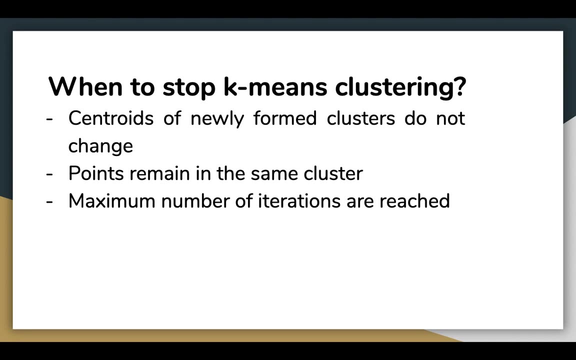 compute the centroids of newly formed clusters. Here the red and green clusters are the new centroids, Step 4.. Now we repeat steps 3 and 4.. So essentially there are 3 ways to stop k-means clustering. First is the centroid of newly formed clusters. do not change. 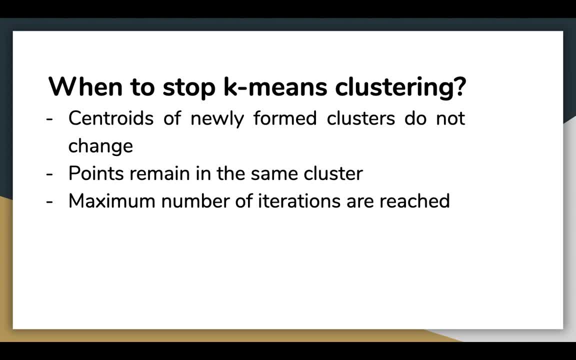 So if the centroids don't change, that means we have reached the end, and that is the best way we can actually cluster our data. Second, the points remain in the same cluster. So if the points remain in the same cluster, that means that there is no further possible. 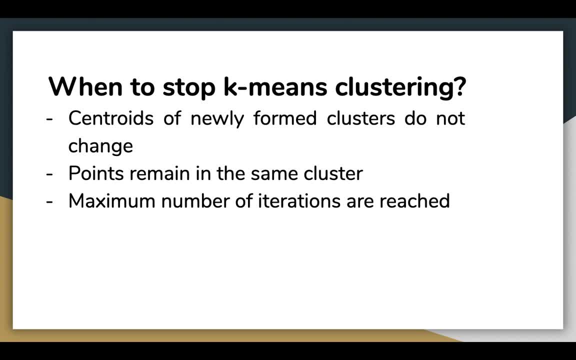 way, or a possible way, to improve our clustering algorithm. And the last is the maximum number of iterations that I reach. So the number of iterations is subjective, so it depends from person to person. So we can actually focus more on the first two points and not on the last point as much.